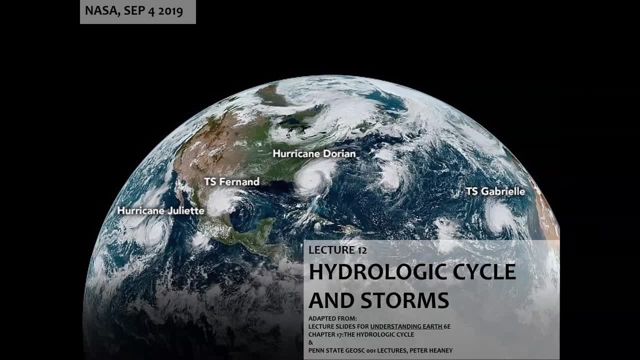 Okay, folks, Today we're going to talk about the hydrologic cycle. Root word there is hydro, meaning water. So we're talking about the water cycle and storms and how those are a part of the water cycle. So in this image of Earth we can see several developing tropical systems. So we've got a tropical storm right here and we've got a hurricane here and a tropical storm over here and a hurricane out in the eastern Pacific. that's headed that way. 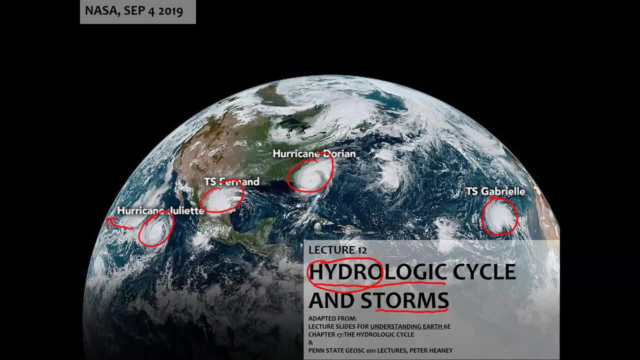 Why so many hurricanes? Why only at one you know specific season during the year do we have those hurricanes? Why are there so many more clouds above this latitude than below, And why is there a relative lack of clouds, sort of in this area here? 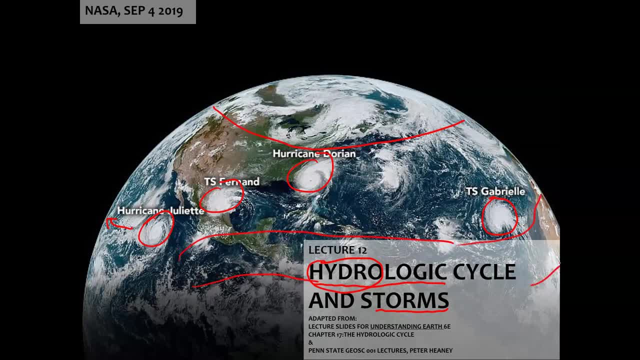 If we looked all the way around, we see there's a desert over there. So how's that related to where there are clouds and where there's water circulating and how air is rising and falling? We're going to talk about all of that today. 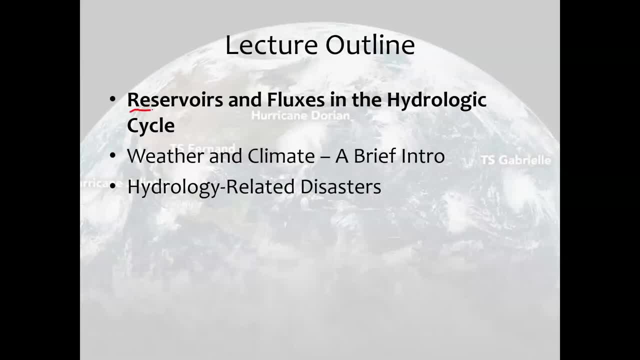 We're going to start by talking about what reservoirs, Reservoirs and fluxes are in the hydrologic cycle, what those words mean and how we determine them and how we can use them to figure out how long water stays in one of a particular place. 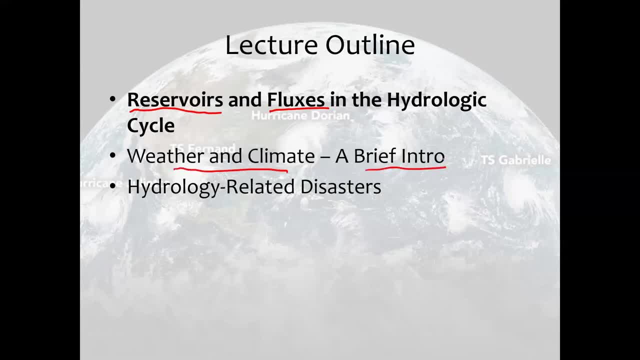 Then we'll talk about weather and climate- just a very brief introduction to it, especially to the weather side of things. And then we'll talk just briefly about hydrology related disasters, in particular hurricanes again. So what are reservoirs and fluxes? 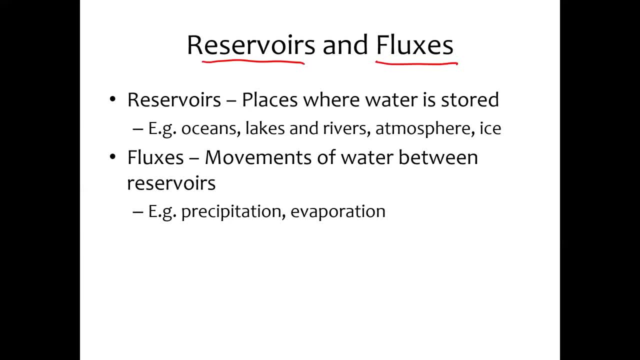 These are terms that describe big picture where water is on Earth's surface. So we can talk about reservoirs that contain water and we can talk about fluxes that move water in between reservoirs. Reservoirs and, put another way, places where water is stored. 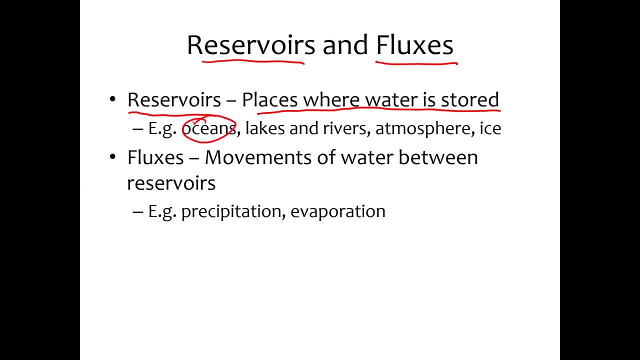 One type of reservoir could be oceans, or lakes and rivers, or the atmosphere or ice, So these are all places that for some amount of time, water is stored And then the fluxes are processes that move water in between those reservoirs: things like precipitation, which would take water from the atmosphere and maybe add it to lakes and rivers, or maybe directly to the ocean, or evaporation, which do the reverse. 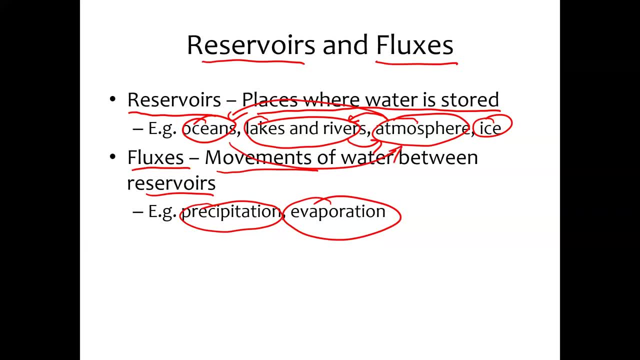 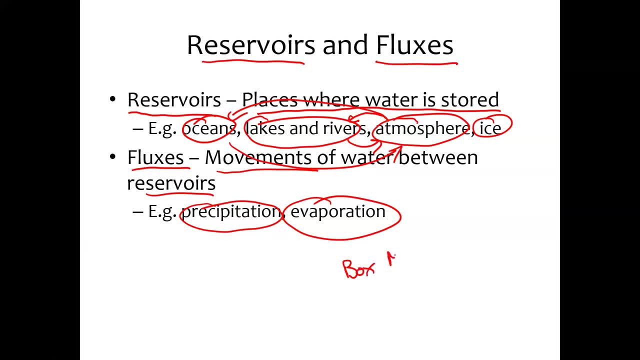 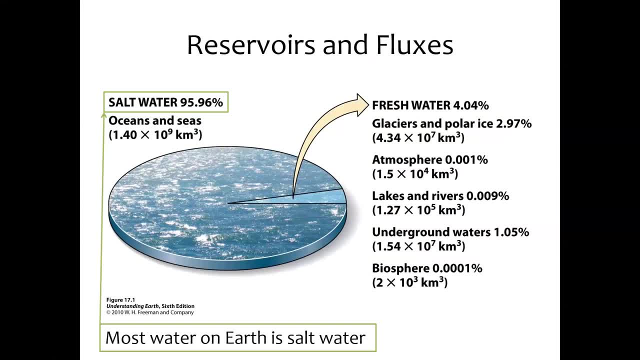 First, let's talk about where on Earth water is stored. So these are reservoirs, right, because we're talking about where water is stored, Most of it on Earth's surface. almost 96% of it is saltwater locked into oceans and seas. 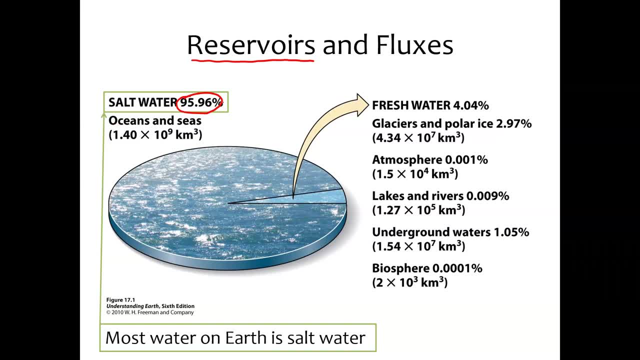 So we can use different units- We can just talk about the proportion of the total- Or we can use different units. We can just talk about the proportion of the total, Or we can use different units. We can just talk about the proportion of the total. 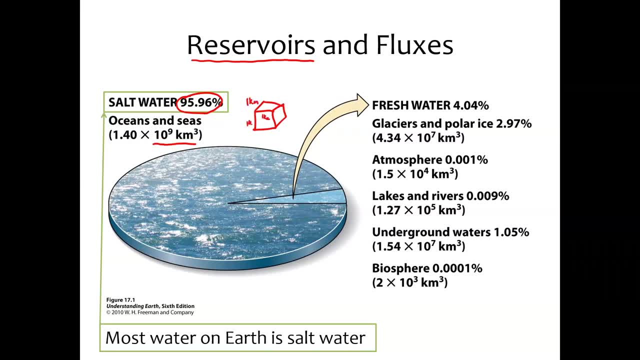 In the sea, we can talk about the number of cubic kilometers. If you imagine a cube, that's one kilometer on every side. that's what that's referring to. In the sea, we can talk about the number of cubic kilometers. If you imagine a cube, that's one kilometer on every side. that's what that's referring to. 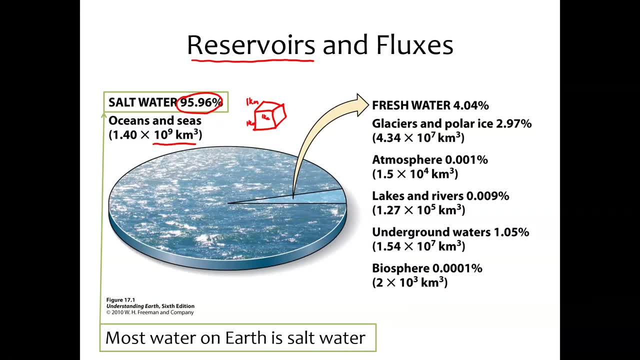 ín Kind of hard to wrap your head around, but it is really just difficult to wrap your head around just how much water there is on Earth's surface, and then that leaves 4% to be freshwater. Most of that freshwater, though, is locked up in ice. 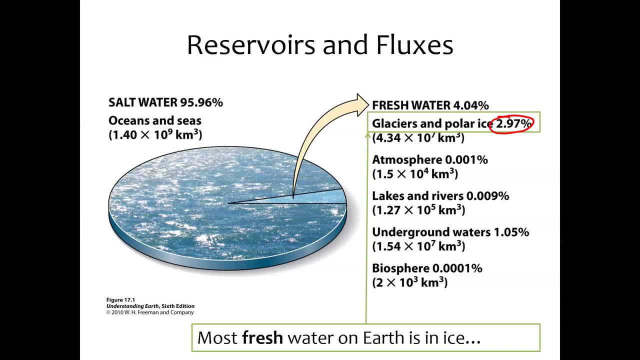 almost 3% out of the whole 4%, so that's nearly three-quarters of all freshwater- is stuck in ice, mostly in the ice sheets that are in Antarctica and Greenland, and then also a little bit locked into other glaciers. For the most part, this is where that freshwater is stored. 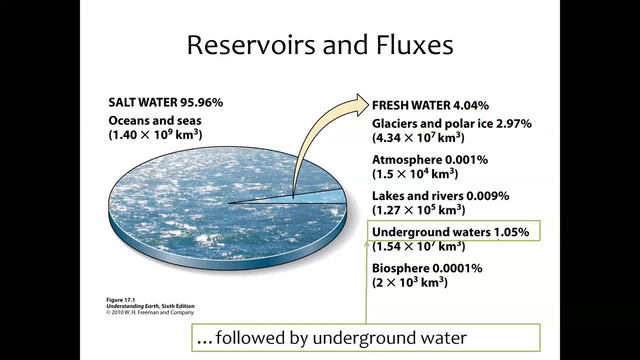 followed by underground water. so water that we could access with a well, say, that counts as underground water and that makes up most of what's left right. so 2.97 plus 1.05% It's going to get. 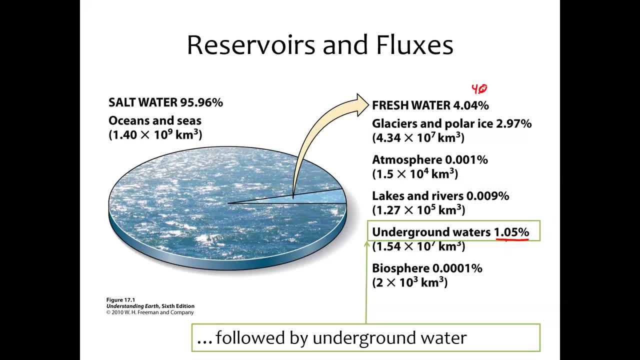 us nearly up to this. It's going to be up to 4.02%. so really that leaves very, very little water for the atmosphere, for lakes and rivers and for the biosphere at any given time. A really small amount is in surface water. 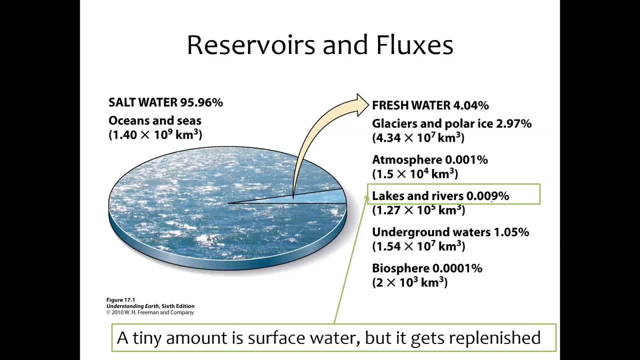 0.009% of all water on Earth's surface is in lakes and rivers at any given time, but it gets replenished rapidly, mostly by precipitation and then addition by groundwater, and so the fact that there's very little water in here doesn't mean we're going to run out of. 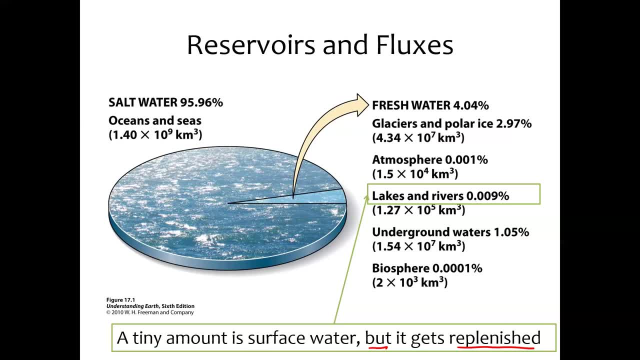 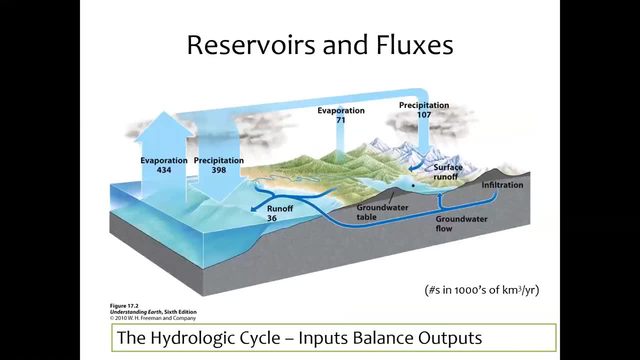 lakes and rivers. It means that they are replenished quickly, and so the water that's in them must circulate through pretty fast. DR MICHAEL armai nie havonske. DJ Wright in Austin, Texas – DR Sque, aquí está el gato. 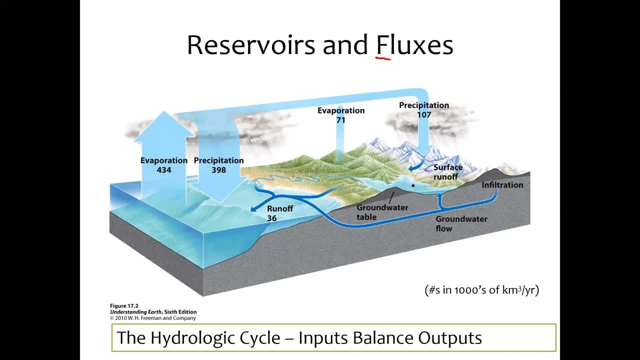 DR. We have changed our, our next parameter now. So here we are changing our view. Before we were looking at reservoirs, the amount in each place. here we're starting to look at fluxes, the amount moving in between each of those reservoirs. and so here these are in thousands of cubic kilometers every year, and 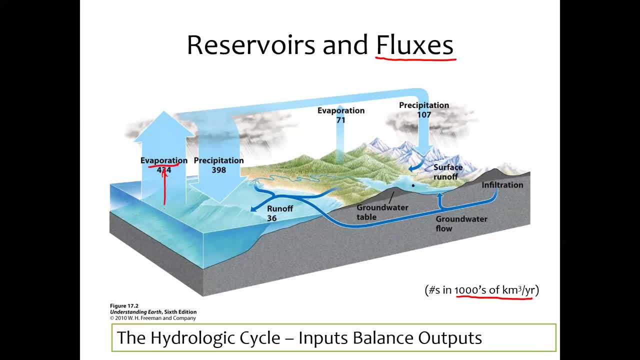 what this means, for example, is that evaporation coming from the ocean- because that's where this arrow is drawn- is equal to 434,000 cubic kilometers every year. That's how much water comes out of the. that's how much water evaporates every year from the oceans, And then some of that rains out as 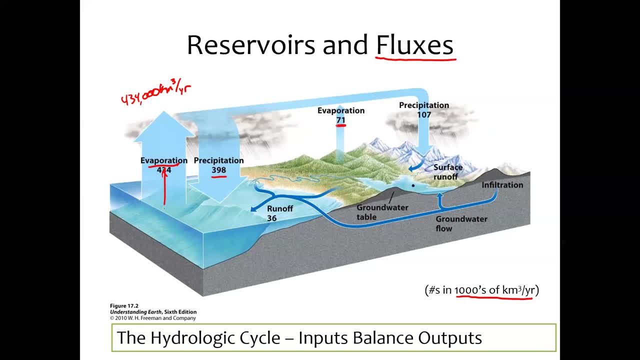 precipitation over the ocean. Then we also have evaporation from the land surface and from lakes and rivers and then precipitation on the land surface. So just looking at these numbers it might look like there's a bit of an imbalance, Like where's the actual water going? More is. 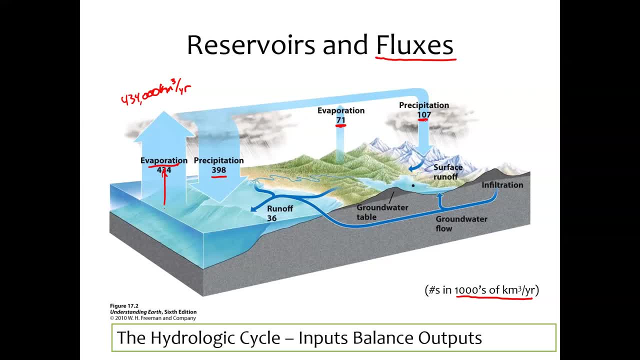 evaporating from the ocean that's running into it, and then more is raining on Earth's surface than is evaporating, at least the solid surface right, the land surface. More is precipitating onto it than is evaporating. So where is the balance? Well, the balance must come in the form of another. 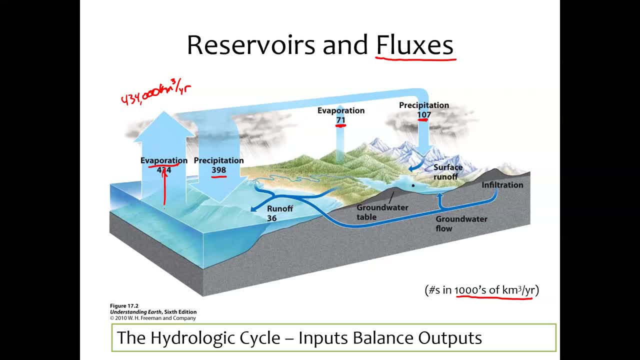 flux. That means that we must take that extra 36,000 cubic kilometers every year, take it from the land surface and move it to the ocean, And that's so that we can balance the total amount of water present in each spot. So that means that runoff is going to both balance the evaporation. 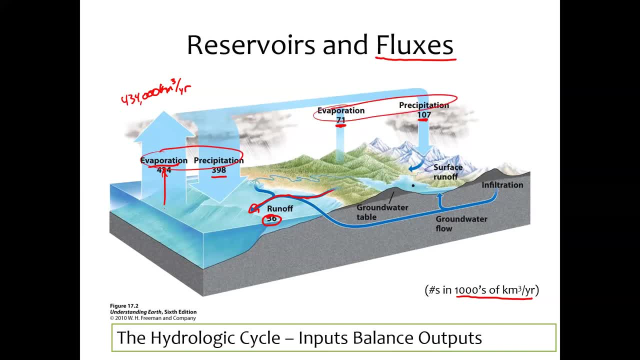 precipitation, and precipitation In the ocean, with the evaporation, precipitation on the land. it means that 36,000 cubic kilometers every year are going to go, run off the land, mostly by way of rivers, and re-enter the ocean. 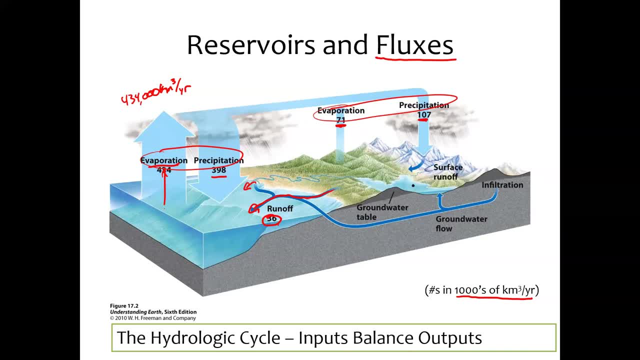 This gives you just a general sense of how much water is moving in between each of these spots, just how much is moving via evaporation, via precipitation and via runoff there, The important thing that I do want to point out is that in a cycle like this, that the inputs really have to balance the outputs on a long 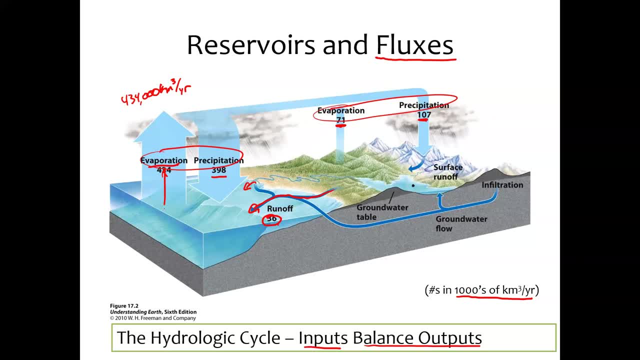 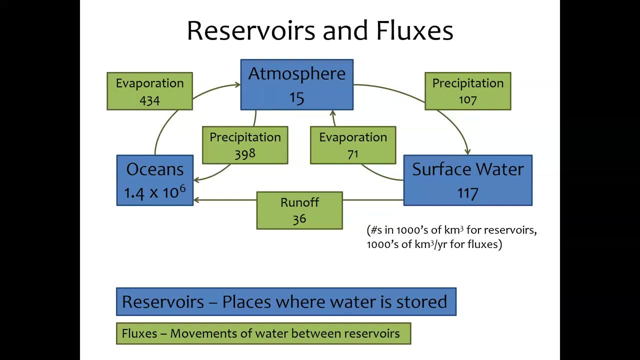 time scale, or else you're going to end up accumulating over and over extra water in one of these places And for the most part, this cycle stays balanced, at least on long time scales over large distances. So here is our box model, where we combine the reservoirs in blue. 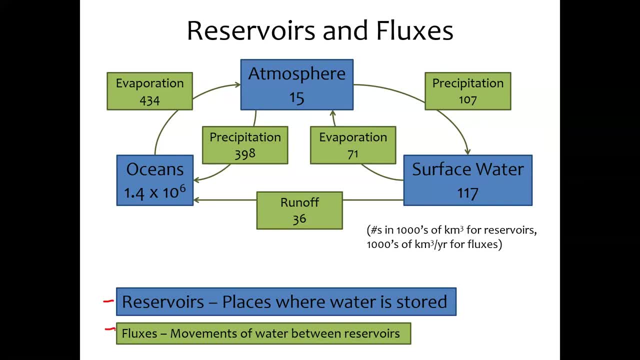 with the fluxes in green and we can start to look at all of the different of the numbers in one spot. so these numbers now are all in thousands of cubic kilometers in the reservoirs, that's just thousands of cubic kilometers total, and in the fluxes, because those 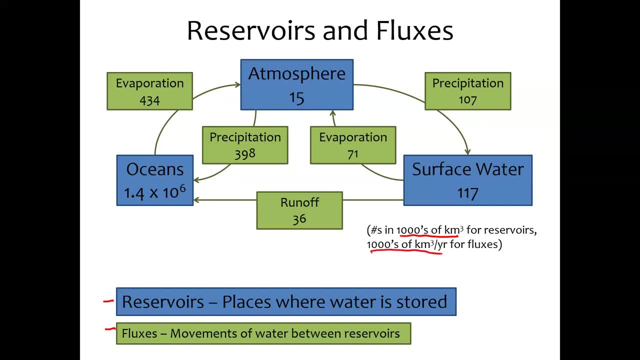 are rates. it's an amount moved every year thousands of cubic kilometers per year. so right, it looks like okay. well, 107 thousand cubic kilometers per year leave the atmosphere to surface water by precipitation, so doesn't it seem like we should run out of water in the? 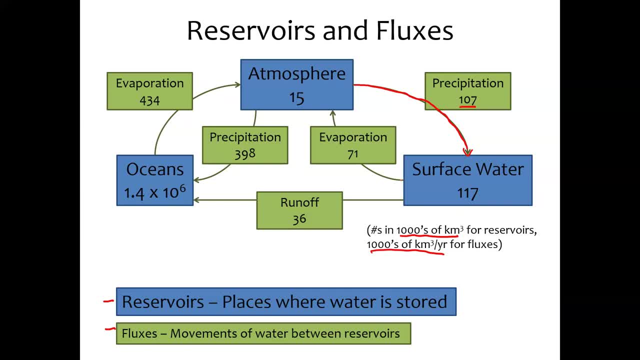 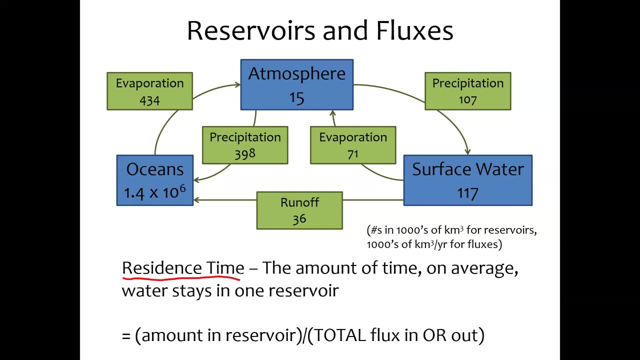 atmosphere pretty fast. well, not exactly, because we're adding more at all times from evaporation from these places- and we can start to use all of these numbers to calculate something that we call the residence time, that is, the amount of time on average- this is definitely an average- water can be. 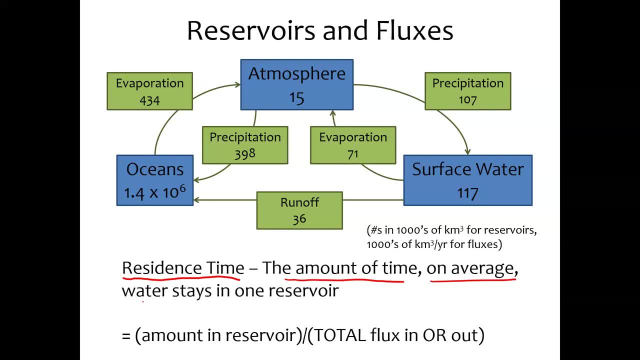 longer or shorter in each of these spots, but it's the amount of time water stays in one reservoir. so the way that we calculate that is we take the amount in that reservoir and then we divide by the total flux in or out, so to figure out the residence time in the oceans. 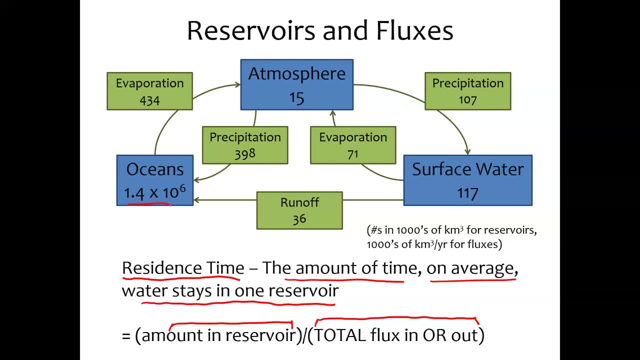 we would have to calculate: okay, we have the amount in the oceans and then we have to know the total amount coming in, that's 398 plus 36, or the total amount going out. in this case, there's only one outflux and that's evaporation, so it should give you the same number if you do that. 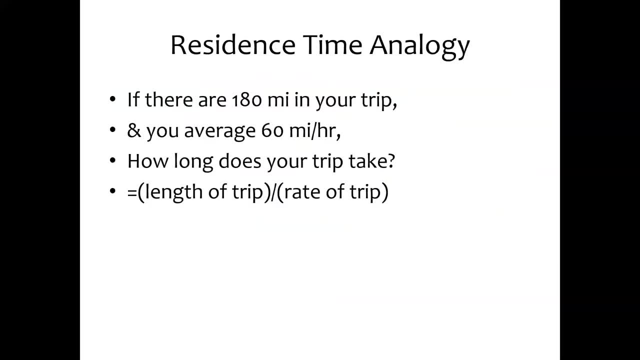 let me give you a little analogy to wrap your head around here. an analogy for residence time would be the amount of time that you're traveling. so you've got a distance which is sort of like the reservoir, and then you've got a rate that you're moving which is sort of like the flux. if there are 180 miles in your 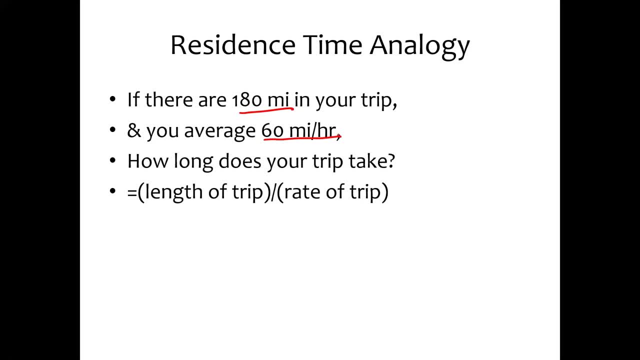 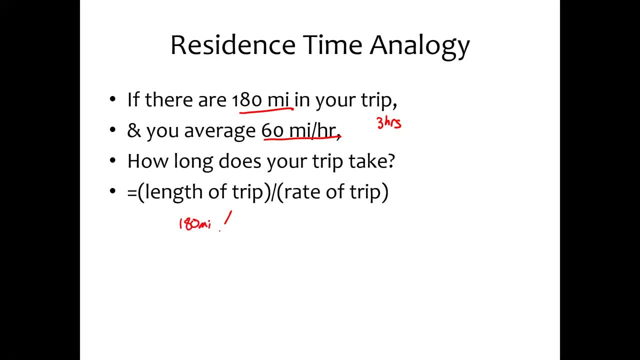 length of trip divided by the rate of the trip and if we do that division it gives us the three hours that we expected to get from that calculation. you're going to do the same thing with the residence time where you're going to take amount divided by flux or rate. 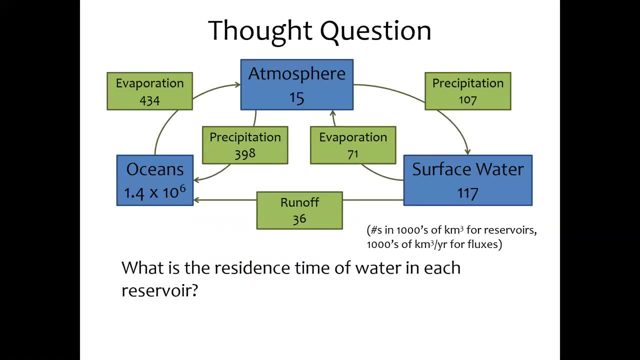 so let's see if we can calculate that for some of these reservoirs. what is the residence time of water in each reservoir? so give it a try yourself with what we just described and then come back and we'll talk about it. let's look at surface water first. so if i do my calculation with surface water, i'm going to start. 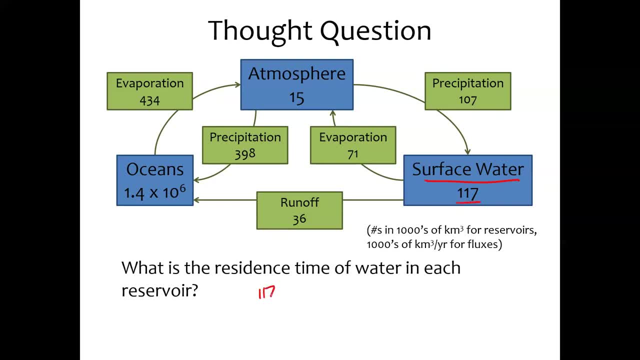 with my 117. so if i have 117 or minus 7 plus 4, and then we can keep the units. you know, if we want to keep the units with it, then we would have to say 117, that's in 1000 cubic kilometers. 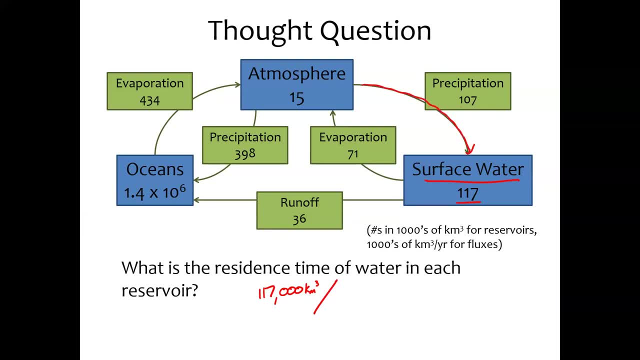 and then we need to divide by the flux, and so we could either use the influx- and this has one influx, so that's probably the best to use- or we can add together both outfluxes. they should give us the same number: does equal 107. So that works. We can use either one, but we have to make sure we use the total. 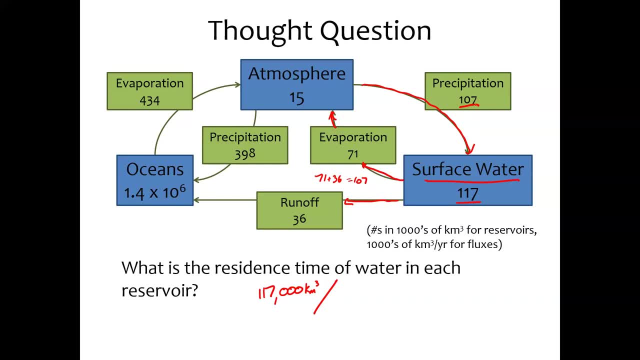 in or the total out. So if there are multiple arrows, you've got to take account for all of them. So we'll take our 107, and that's in. what are the units there? It's thousands of cubic kilometers per year, And this helps us keep track of what the units are going to be when we do this. 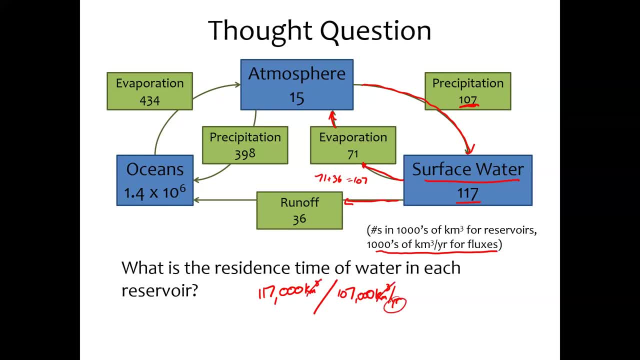 division. Cubic kilometers will cancel out and then the years will end up on top. So this is going to be a time in years. So if you do 117 divided by 107, you should get a number of about 1.09,. what are the units? Years. So on average, in surface water, that water will stick around. 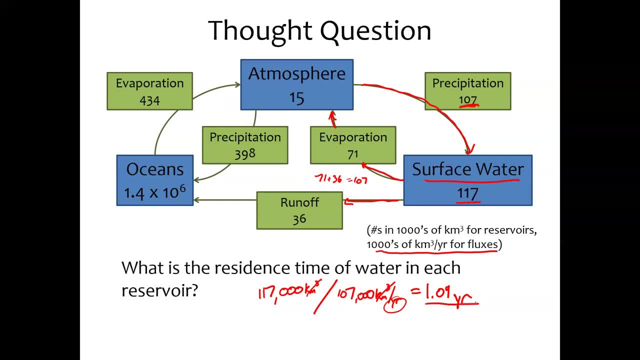 on the surface for a little over a year. That takes into account the fact that some water is going to fall right at the end of the Mississippi River and it's going to enter the river directly and end up right back in the ocean. So that's going to be a time in years. So if you do, 117. kilometers per year, that water will stick around on the surface for a little over a year. That takes into account the fact that some water is going to fall right at the end of the Mississippi River and it's going to end up right back in the ocean right away, So some of it might only be. 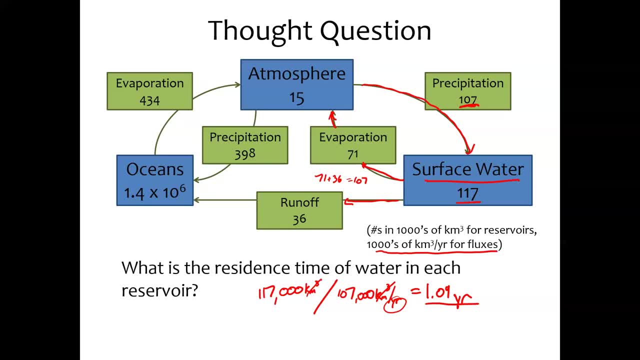 there for a few days or even hours, And then some water might land somewhere very far upstream and take a really long time to percolate downward through the soil and out into the river and take years to reach it. So if you average all that together, you get that water and surface water. 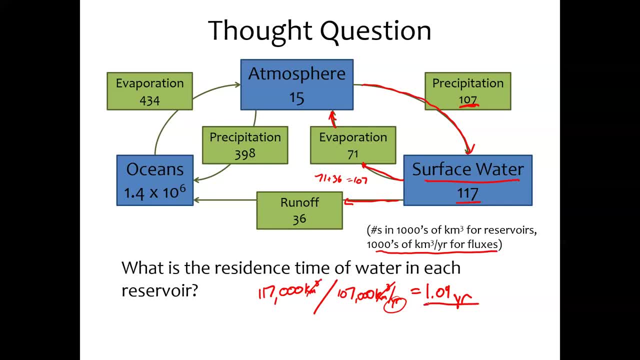 sticks around for about 1.09 years on average, a little more than a year. What about oceans? This is tricky a little bit because it's got the scientific notation in there. So if we write it out, we're going to write 1, and then we're going to write 4, and then we're going to put some zeros on. 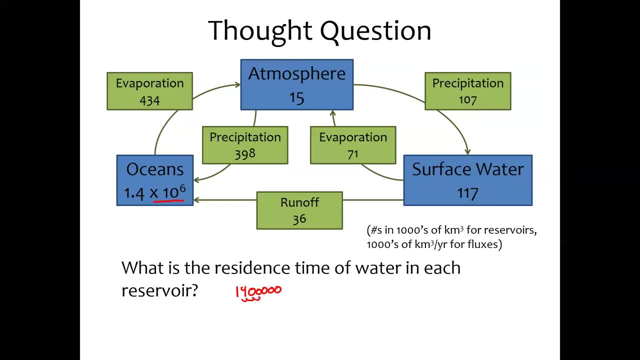 there Say 1,, 2,, 3,, 4,, 5,, 6.. And then we remember that this is in thousands of cubic kilometers per year. so add another three zeros on there. Excuse me, this is just in cubic kilometers because it's. 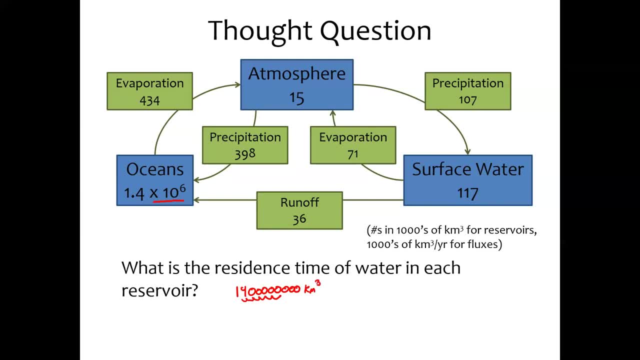 a reservoir. And then we've got to figure out, okay, what is the flux. So we could either use one flux out as 434 or two fluxes in added together, You give us the same number, so that's good. So we divide by 434,000 cubic kilometers per year. So making sure that we are careful, 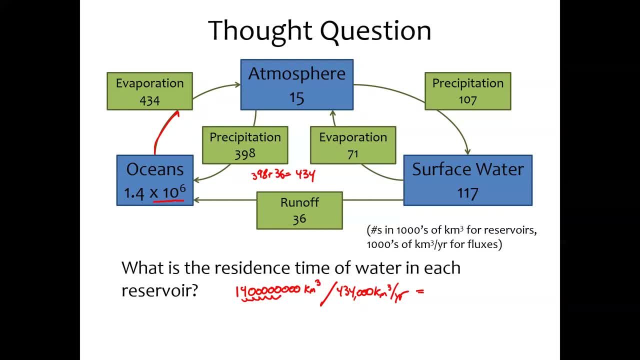 to keep the right number of zeros in there. I get remembering that we should have only so many significant figures in here. an answer of about 3,200 years. So that means that on average, water that is in the ocean is going to stick around for.